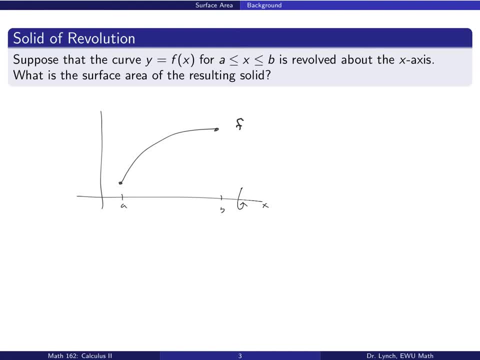 revolving that chunk of a curve around the x-axis. So we'll start off with some preliminaries here and sort of build up our intuition on what that surface area should be. Here's the first preliminary. Let's go ahead and think about a cone with radius r. 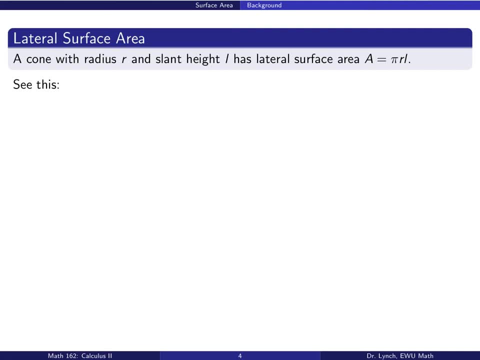 and slant height l, It turns out that the lateral surface area- so when I say lateral surface area I don't mean the surface area of the end, but just the cone part- is pi r l. So we can see this pretty quickly with just a little bit of geometry. So if we think about the lateral 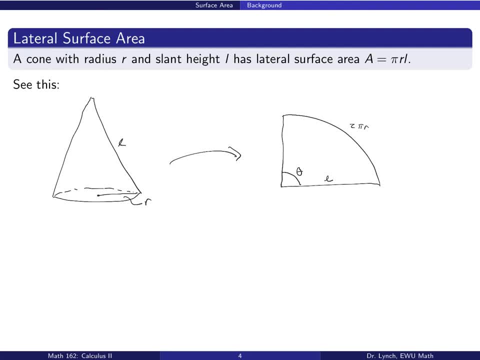 surface area. again, I'm not thinking about the end of the cone here, but just the lateral surface area of this cone. we can try to find that by slicing open our cone, laying it flat, and when you do that you can see that the cone is a little bit more flat. So we can try to find that by 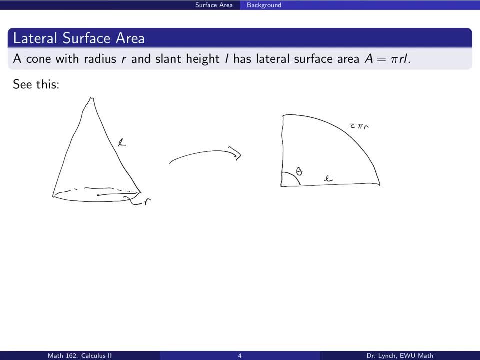 slicing open our cone, laying it flat, and when you do that you can see that the cone is a little bit more flat. So we can imagine that you'll sort of have the sector of a circle here and that sector of the circle will. 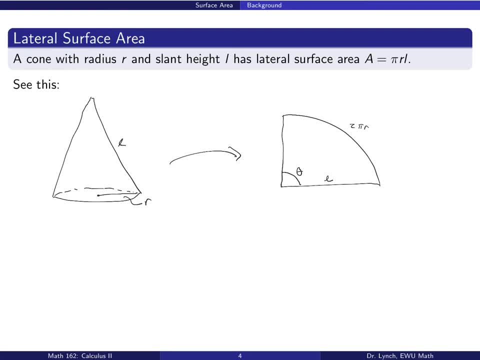 be some sector with length l for the radius and angle theta which sort of matches that arc of the circle to pi? r. Now we know a couple of things here. The first thing we know is that that arc is related to the angle of the sector of the circle by the equation: 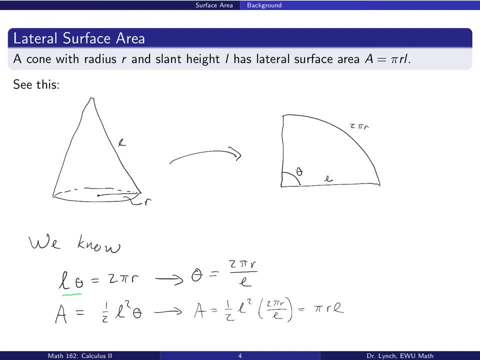 l, theta equals 2 pi r. So this allows us to write theta in terms of r and l, as theta equals 2 pi r over l. Now the other thing we know is that when we have a circle with radius, in this case l. 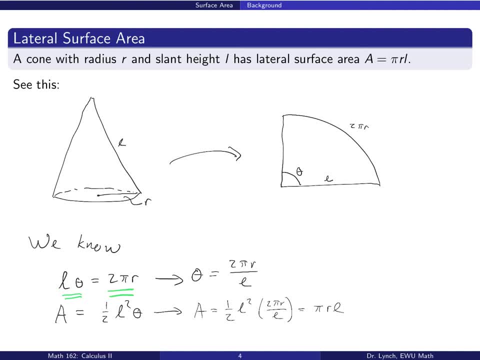 and angle theta, that the area of that sector of a circle is given by the angle theta. So we can imagine that the area of that sector of a circle is given by 1 half l squared theta. Substituting our expression here for theta, we can identify that the area is exactly pi? r l, just like I promised. 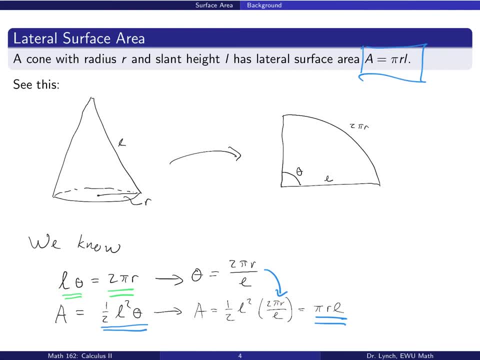 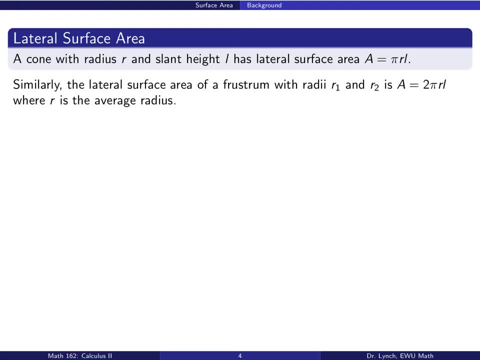 Okay, so the area of that cone is pi r l. Now we can use this to find the lateral surface area of a frustrum defined by radius r1 and r2.. And we do that just by thinking about taking the difference of the surface areas of two cones. 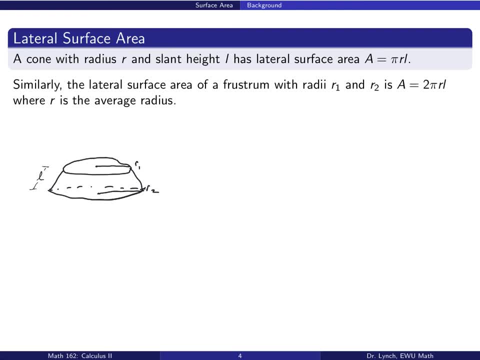 So here's our frustrum, with slant length l, radius r1, radius r2.. And in order to think about the surface area of that frustrum, we'll go ahead and extend it up so that it becomes a big cone. Here's what that looks like. So here we've extended. 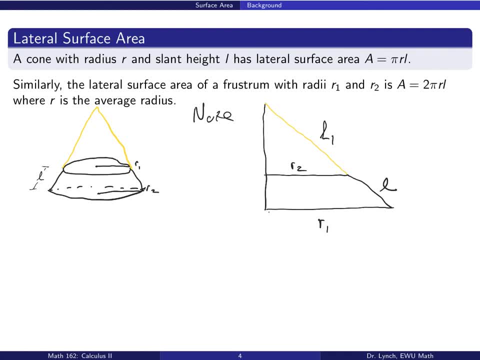 our cone, up our frustrum, to make a giant cone, And I've sort of taken a cross-section of that. that ends up being a triangle with two bases: r1 and r2.. And there are a couple different lengths here: l 1, and l. Now we can use special triangles to relate l1 to our other measurements. 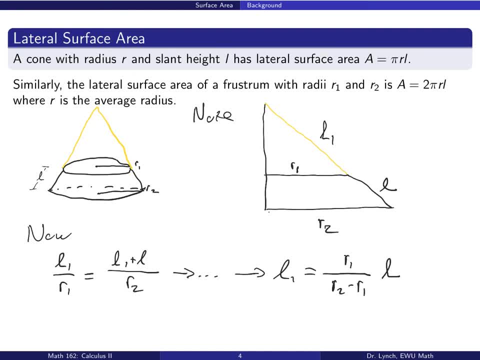 So here's that relationship. I had previously mislabeled r1 and r2.. So that's fixed now by similar triangles. l1 over r1 is equal to l1 plus l over r2.. We can solve for l1 in terms of r1,. 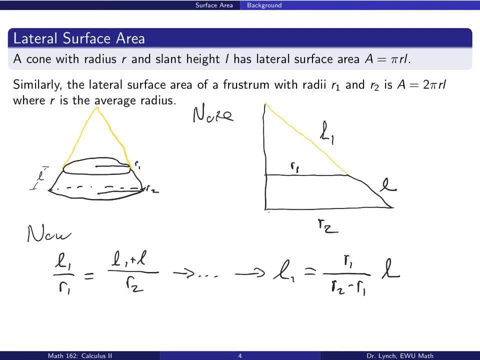 r2, and l, And this allows us to write the area of the frustrum as the difference of lateral surface areas of two cones. Okay, and again, my strategy here is to write the area of the frustrum as the area of the big cone, And then I'm going to go ahead and add this area of the big cone And 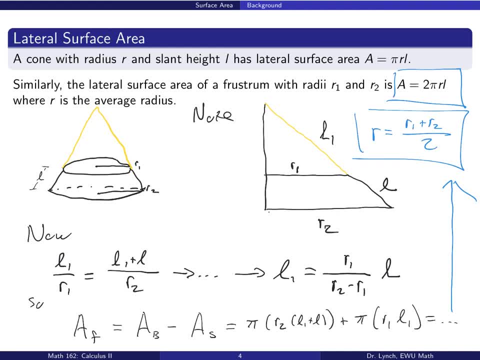 I'm going to go ahead and add this area of the big cone And I'm going to go ahead and add this area minus the area of the little cone. The area of the big cone is pi times R2 times the big length, L1 plus L. The area of the little cone is pi times R1 times. 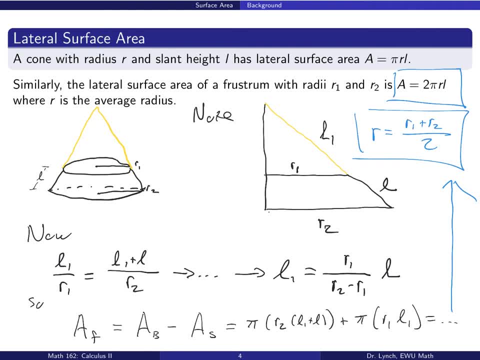 L1.. Simplify, simplify, simplify. Write R as the average of the radius R1, plus R2 over 2, and we get the area of the frustrum 2 pi RL. Again, R here is the average radius. Okay, so that's a lot of background, but this frustrum lateral. 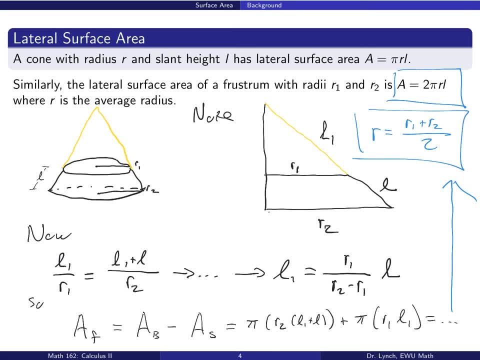 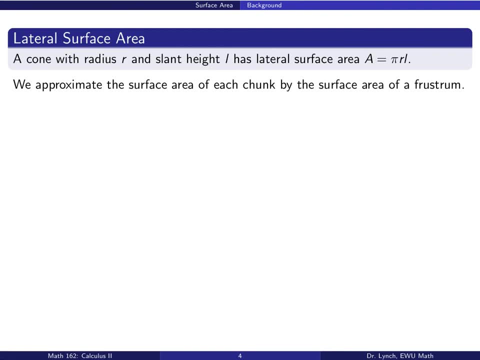 surface area is what's going to end up giving us the surface area of one of these volumes of revolution. Here's what it looks like If we take our curve and wrap it around the x-axis and think about surface areas of chunks of that curve. 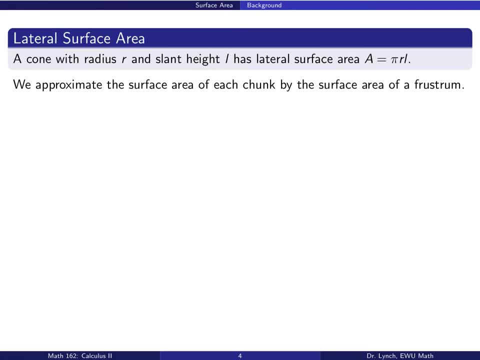 we can approximate that surface area of each chunk by the surface area of a frustrum. So here again I've drawn just some random curve f of X from A to B. Let's think about just a small chunk. So in other words, we're, as usual, divide an. 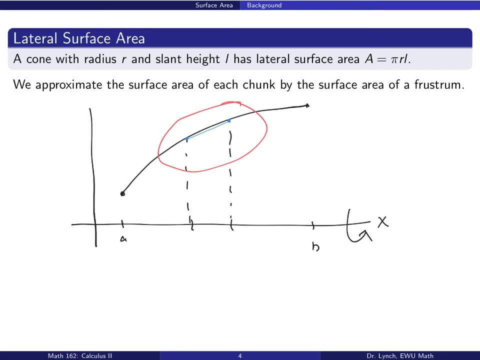 interval from A to B into subintervals of equal width, Delta X. and then think about revolving that piece, zooming in and you can imagine that the surface area connecting those blue dots is approximated by the surface area of the frustrum and the area of the frustrum of a frustrum. 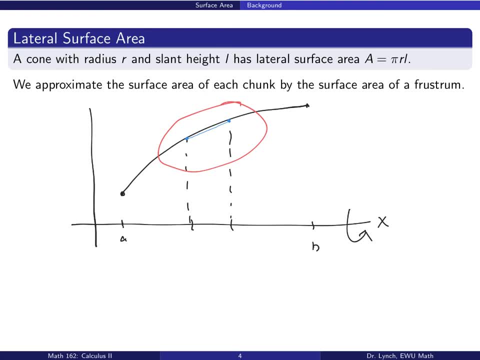 area of a frustum and that frustum has has average radius given by f of X. I star for somewhere in between- and the lateral length is exactly the arc length. here's what it looks like and I'll go ahead and express this in terms of differentials. so here are a little bit of surface area D. capital S is 2 pi. 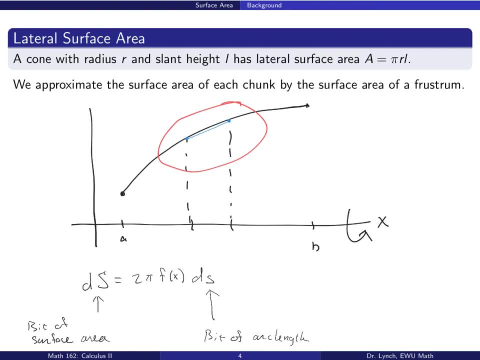 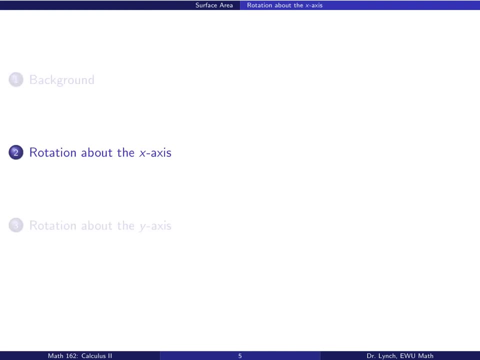 times f of X, times a little bit of arc length DS and depending on the formulation of the problem, like we talked about last time, we may prefer to express that arc length in terms of functions of X or maybe functions of Y. so again, let's go ahead and think about rotation around the x-axis. we'll do this. 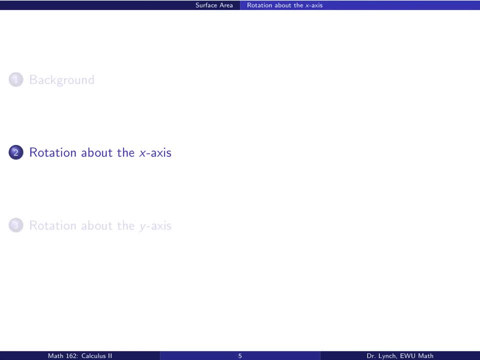 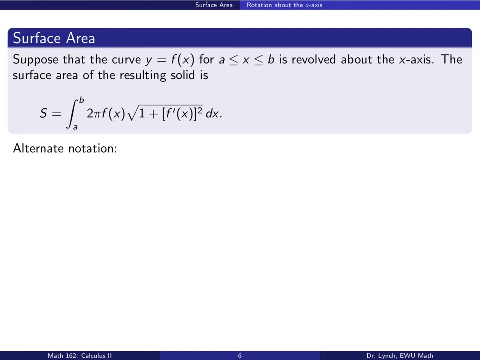 sort of quickly thinking about adding up circumferences of circles along the arc length. so if we have the curve, y equals f of X for a less than equal to Lexus, X, less than equal, to be revolved around the x-axis, the surface area, the resulting solid is the integral. 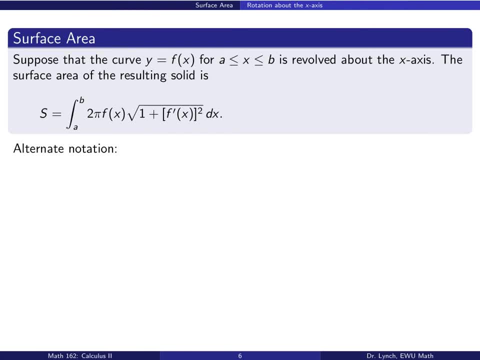 from A to B of 2, pi, f of X times the square root of 1 plus f prime of x squared DX. and here's our alternate notation. so again, we'll sort of stylize this surface area as adding up circumferences of circles along an arc length. now the 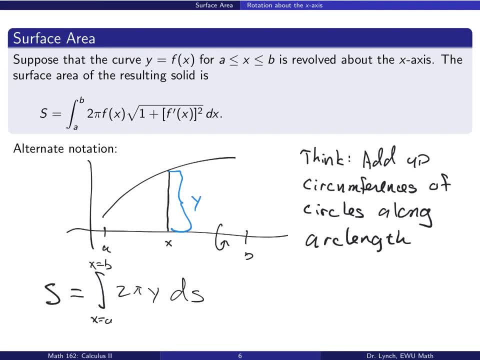 circumferences of the circles have a radius Y. so we're thinking about adding up these circumferences of circles given by 2 pi y. those are the circumferences along the arc length DS, from X equals A to X equals B. and then, if we know that, 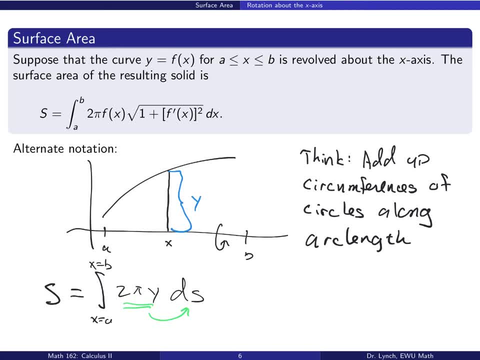 Y is f of X and we know that the arc length is the square root of 1 plus f prime of x. we can quickly see how we end up with the integral from A to B of 2 pi f of x times this unit of arc lengths, which is the square root of the quantity 1 plus f. 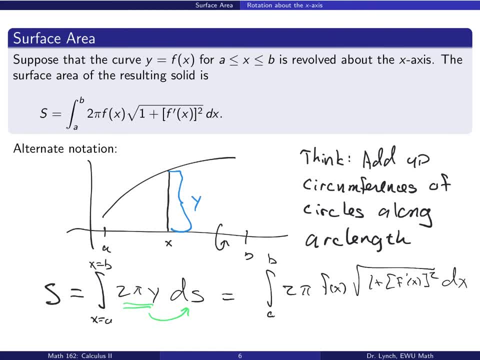 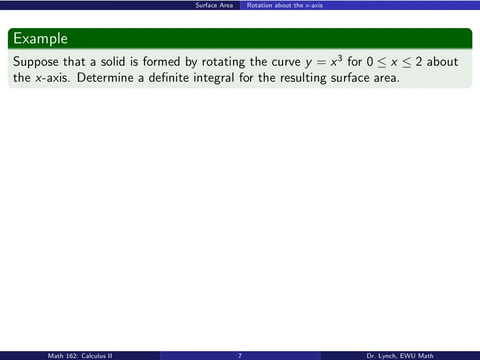 prime squared DX. ok, here's an example. suppose that we rotate the curve. Y equals X, cubed for 0 to 2 about the X axis. let's just go ahead and write down a definite integral. we won't evaluate it for the resulting surface area. pictures are nice. 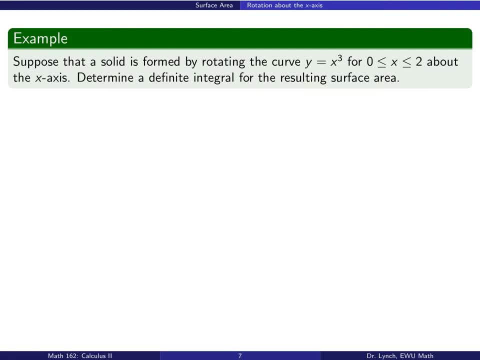 are nice. we'll start off with the picture and then again we'll think about adding up circumferences of circles along the arc length. so again here, y is x cubed. we're adding up circumferences of circles with radius y along the arc length dx, and in this case, 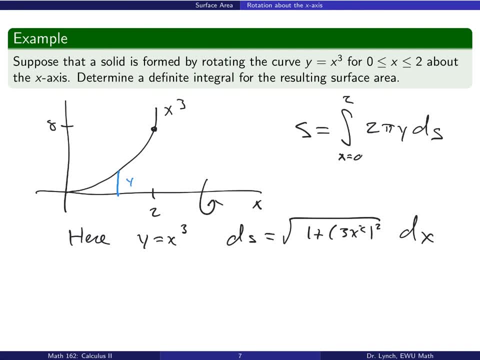 that arc length unit is 1 plus the square root of 1 plus 3x squared squared dx. so here's a perfectly good, definite integral expression for our arc length: the integral from 0 to 2 of 2 pi x cubed times the square root of 1 plus 9x to the fourth dx. now it turns out that this is an integral that. 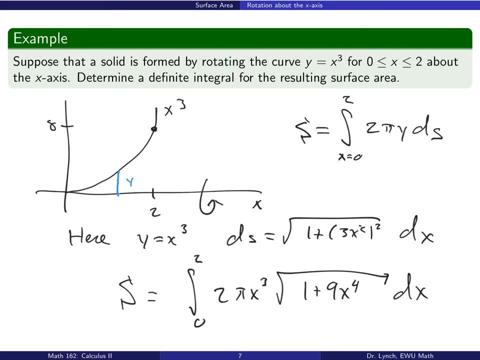 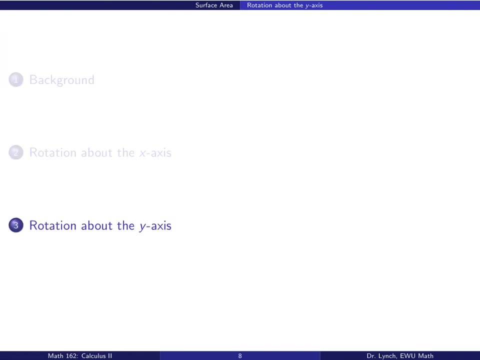 we can evaluate just with a u substitution. i won't go through that here, but it's not so. it's not so bad. and again, here i'm thinking of this as surface area. so surface area with a capital s to avoid confusion with arc length with a little s. okay, so let's go ahead and talk about rotation around. 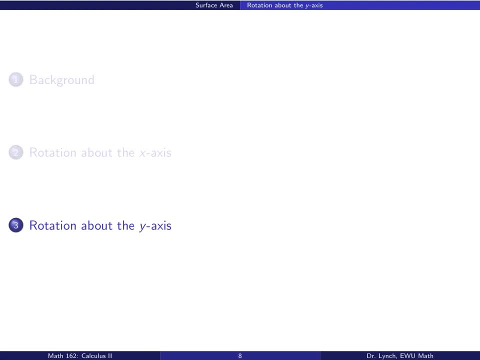 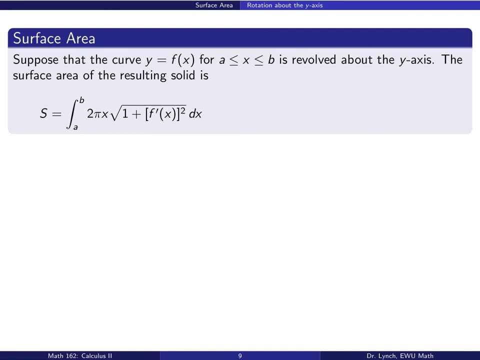 the circle. so let's go ahead and talk about rotation around the circle. so let's go ahead. and y-axis, and the idea is sort of similar here. it turns out when you rotate around the y-axis that the area of the resulting solid is 2, pi x times 1 plus f, prime of x, squared all square root of dx. 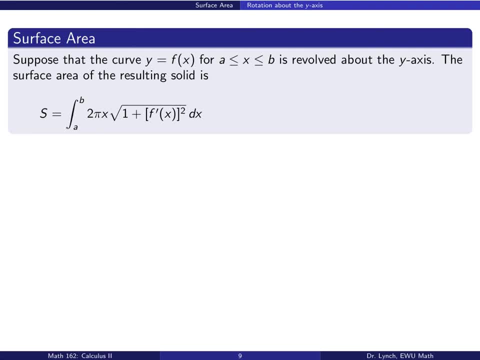 and again. we can think about this in terms of adding up circumferences of circles along the arc length. the only difference is, in this case, the circumferences of those circles are given by 2 pi x instead of 2 pi y. so once we identify that this arc length unit is given by